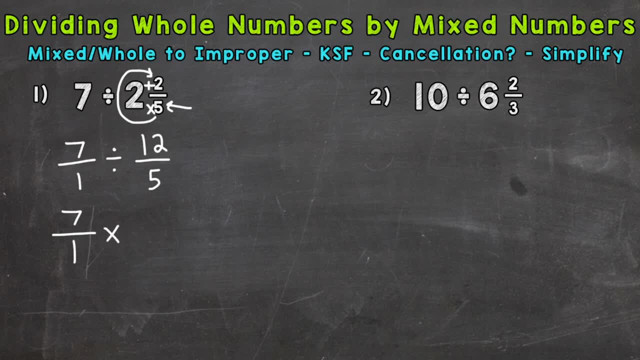 We're going to do a multiplication, That means we need to flip our second fraction. So the 5 is now our numerator and the 12 is the denominator. So now we're ready to solve and multiply straight across. But before doing so we can always check to see if we can use cancellation. 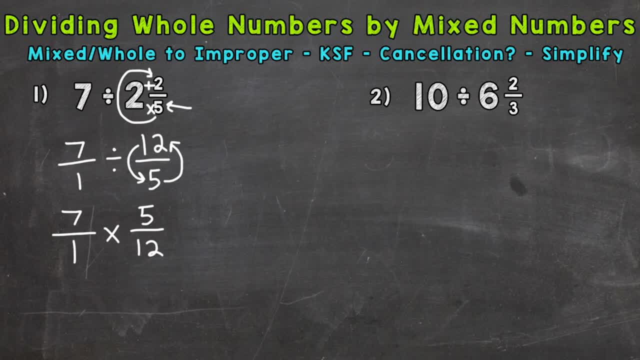 So you can think of this as simplifying the problem before multiplying straight across. So what we need to do, we need to look for common factors between our numerators and denominators. But in the case of number 1, the only common factor between our numerators and denominators is 1.. 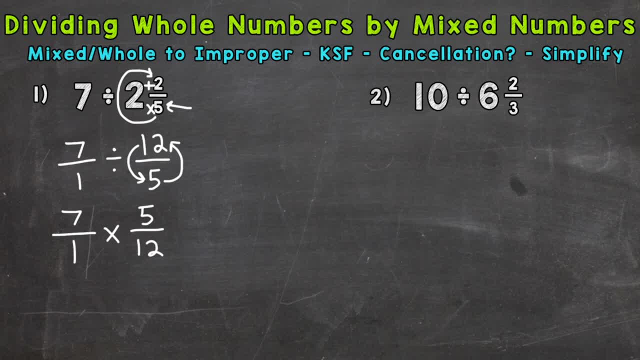 So we can't use cancellation for number 1.. We will be able to in number 2, but we'll get there in a minute, So we can multiply straight across now: 7 times 5 is 35. And 1 times 12 is 12.. 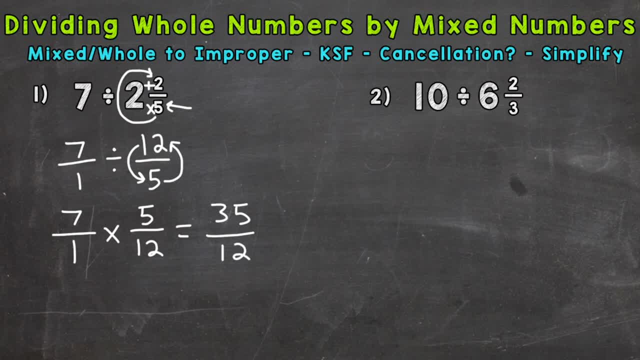 So we can multiply straight across now. So 35 over 12 is our final answer, but it's an improper fraction, So we want to convert it back to a mixed number. So we do that by doing 35 divided by 12.. 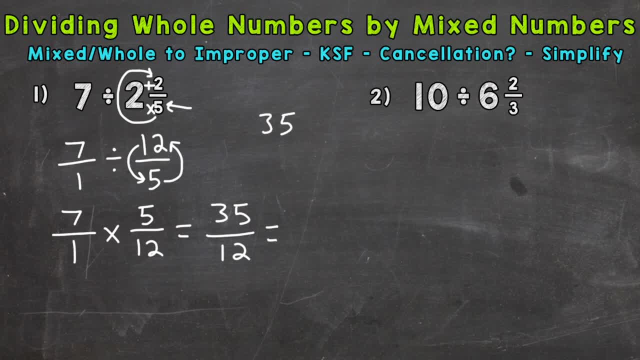 So let's actually write all of this out. So 35 divided by 12.. So how many whole groups of 12 can we pull out of 35?? Well, only 2. That gets us to 24, because 3 groups, we would need 36.. 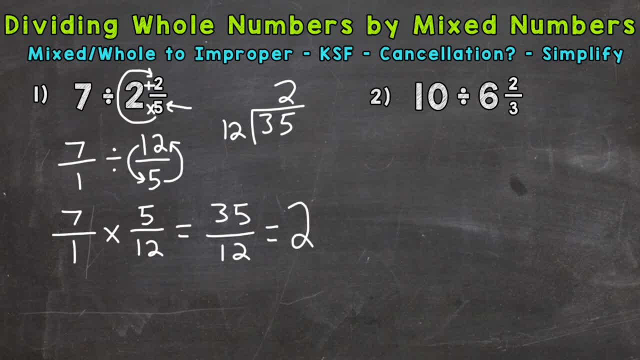 So 2 whole groups, that's going to be our whole number portion of the mixed number. So 2 times 12, 24.. Subtract we get a remainder of 11.. So that remainder is going to be the numerator of our fractional part. 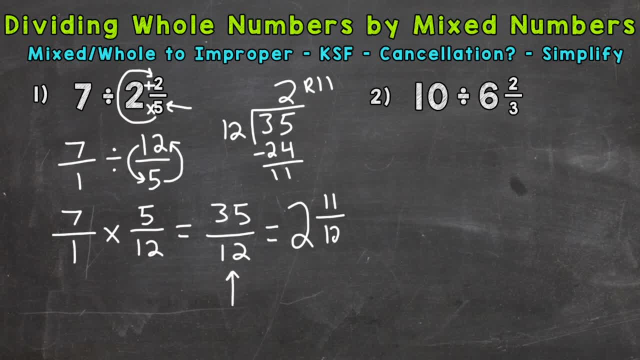 And then we keep our denominator of 12 the same. Always check to see if you can simplify the fractional part. 11, twelfths, only common factor between the 11 and 12 is 1.. So we are in simplest form. 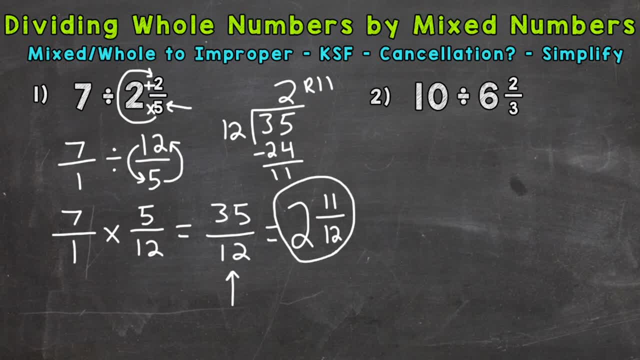 And our final answer is 2 and 11 twelfths. So on to number 2, where we have 10 divided by 6 and 2 thirds. So first thing we want to do, convert our mixed number and whole number to improper fractions here. 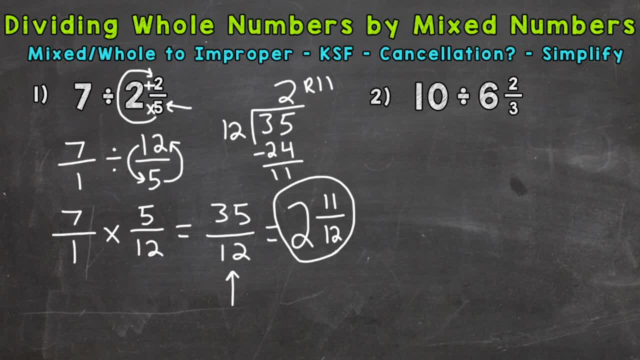 Or put in fractional form. So the 10, the whole number we can put over 1. Bring our division sign down. So mixed number to improper, we start at the bottom, We multiply and then add. So 3 times 6 is 18, plus 2 is 20.. 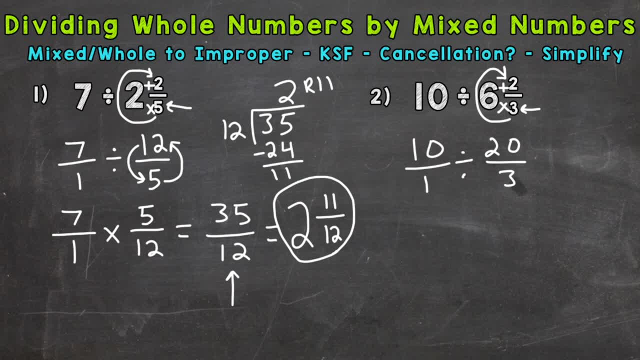 Keep our denominator of 3 the same. So now we're ready to keep switch flip. So always keep your first fraction, Switch and then flip, So we have 3 over 20.. Now we are ready to multiply straight across. 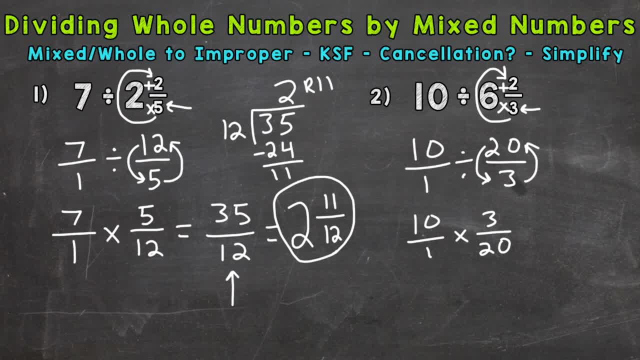 But we can look for cancellation. And in the case of number 2, we do have a common factor between our numerators and denominators. So if you look at the 10 and the 20, we have a greatest common factor of 10 between those two. 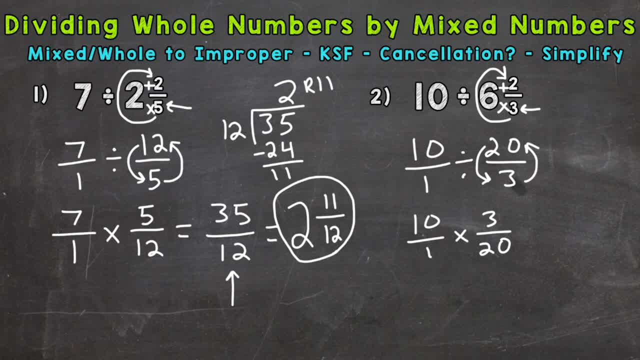 So we can divide both of them by 10.. Before we multiply straight across Again, think of cancellation as simplifying the problem before multiplying straight across. So let's divide 10 by 10 and 20 by 10, our greatest common factor between the two. 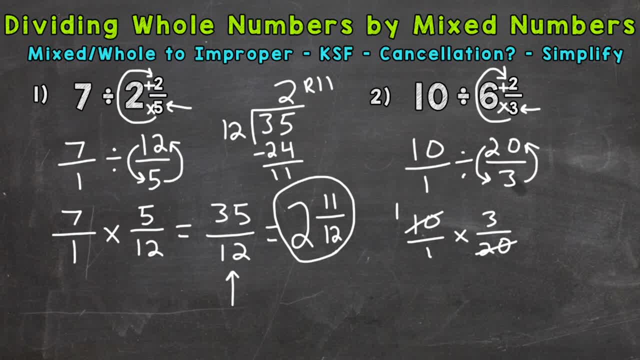 So 10 divided by 10 is 1, and 20 divided by 10 is 2.. So now we can multiply straight across: 1 times 3 is 3,, 1 times 2 is 10, 2.. So we end up with an improper fraction, and that is our answer. but we always want. 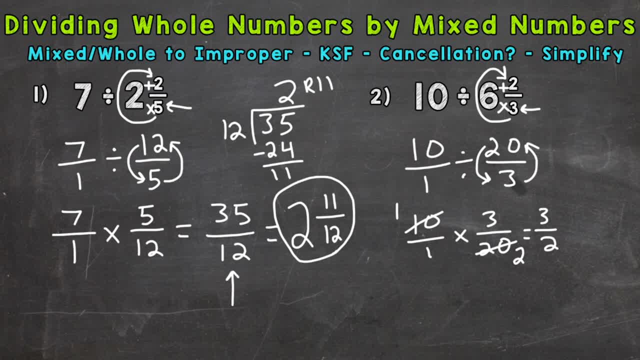 to change our improper fraction answers to mixed numbers. for our final answer, So 3 halves, or 3 over 2, we need to do 3 divided by 2 in order to convert this to a mixed number. So how many whole groups of 2 out of 3?? Well, 1.. And we have a remainder of 1, and we can. 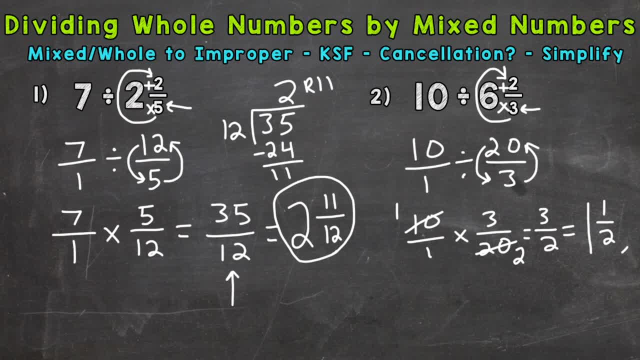 keep our denominator of 2 the same, So we end up with 1 and 1 half there. Always check to see if you can simplify the fractional part of a mixed number. but 1 half is in simplest form. so we are done and our final answer is 1 and a half. Now I do want to show you. 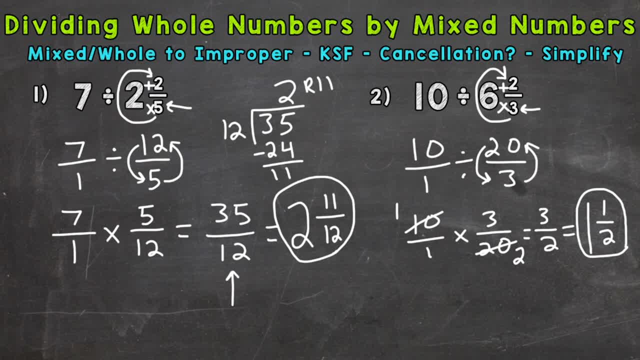 a comparison here between using cancellation and not using cancellation. So I'm going to rewrite the problem. We have 10 over 1 times 3.. We have 20 over 20.. So let's see what answer we would get if we didn't use cancellation. 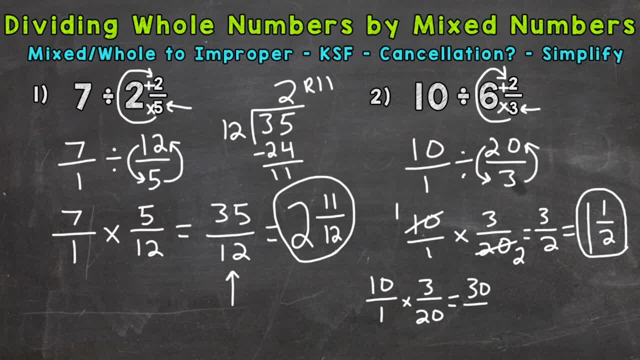 So 10 times 3 is 30, and 1 times 20 is 20.. So we get 30 over 20.. Again, that's an improper fraction, just like we had with using cancellation. so we want to convert that to a mixed number. 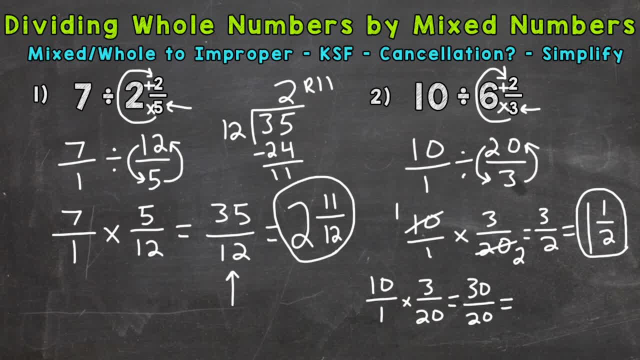 So 30 divided by 20.. How many whole groups of 20 can we pull out of 30?? Well, 1 with a remainder of 10.. And we keep our denominator of 20 the same. So we end up with 1 and 10. twentieths Now. 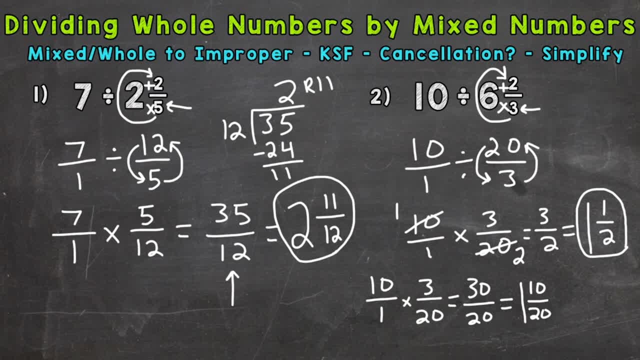 that fractional part we can simplify. The greatest common factor between 10 and 20 is 10.. So let's divide each by 10 here and we end up with keep our whole number of 1 the same: 10 divided by 10 is 1,. 20 divided by 10 is 2.. So we end up with the same number. 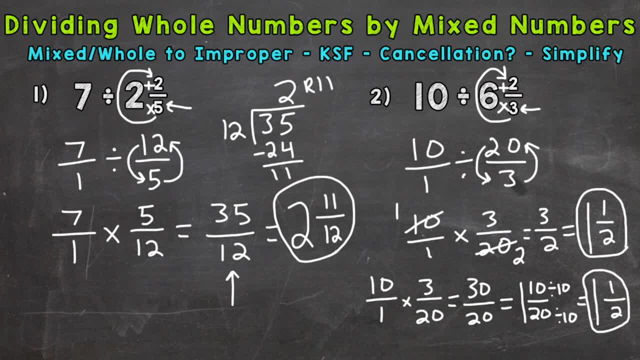 of 1 and a half. We just simplified at the end rather than before. we multiplied straight across. So, whether you use cancellation or not, you will end up with the same answer. just a couple of different paths in order to get to it. 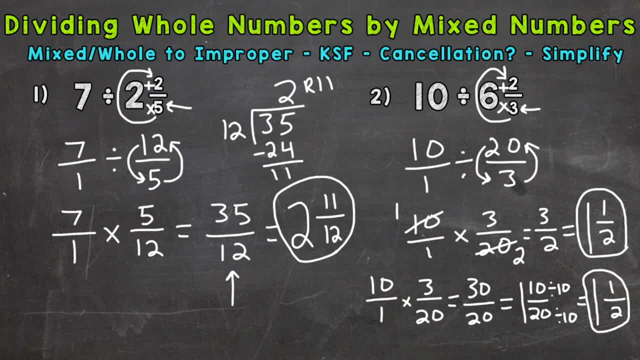 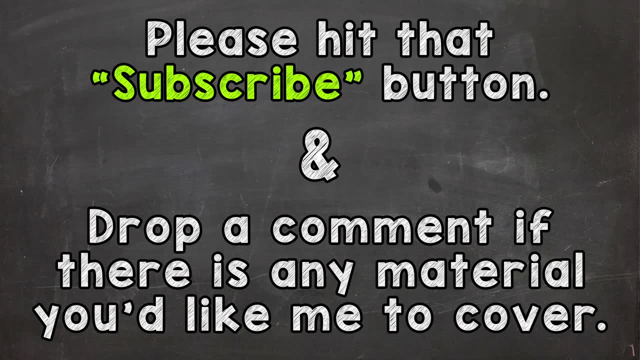 So there you have it. There's how you divide whole numbers by mixed numbers. I hope that helped. Thanks so much for watching. Until next time. peace Subtitles by the Amaraorg community.